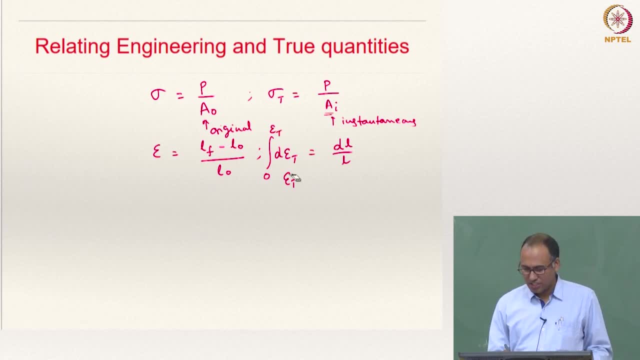 to whatever strain that you are interested in, then this will be epsilon t. that will be equal to integral initial length, final length, dL over L, that is natural log integral l divided Lf by L0, right, That is the definition of your proof string. all right, Now, if I were, 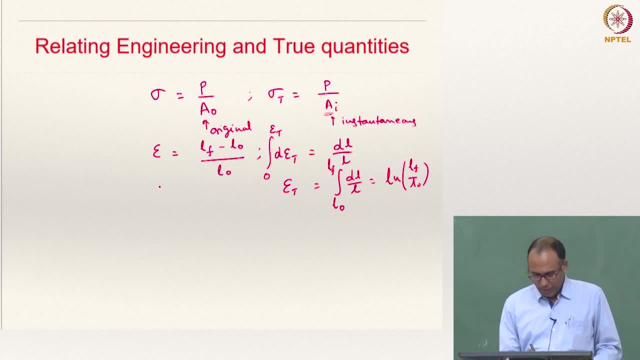 to. so this, so epsilon can be written as Lf by L0 minus 1 or 1 plus epsilon is equal to Lf by L0, right, So that implies I can write: my true strain is equal to natural log 1 plus epsilon, because this quantity is basically this and that is how your true strain and 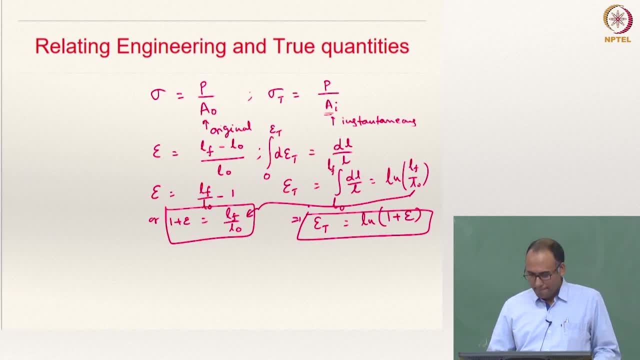 engineering strain are related. all right, Now let us try to relate the proof string, The true stress and engineering stress. So we know that true stress equal to P by Ai. So if I multiply this guy with A0 and divide this with A0, then I have P by A0 times A0. 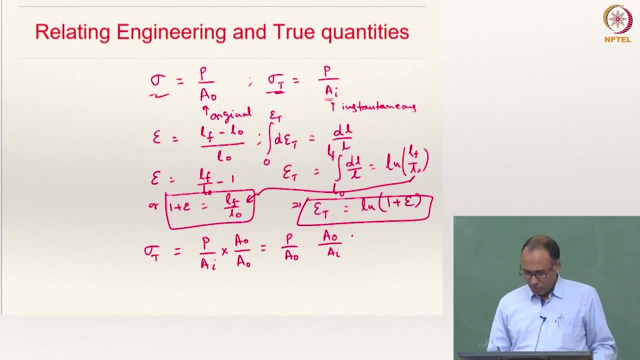 by Ai. okay, So P by A0 is what? That is our engineering stress. I am not writing anything as a subscript to sigma. Okay, So P by A0 is what. That is our engineering stress. I am not writing anything as a subscript. 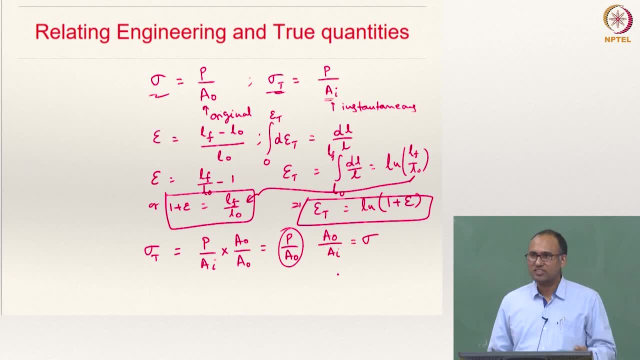 to sigma when it is an engineering quantity. If it is a true quantity, then I am writing subscript T. okay, That is how you recognize times A0 by Ai. And now we have discussed about the volume constancy condition, which means A0, L0 must be equal to Ai Li, okay, 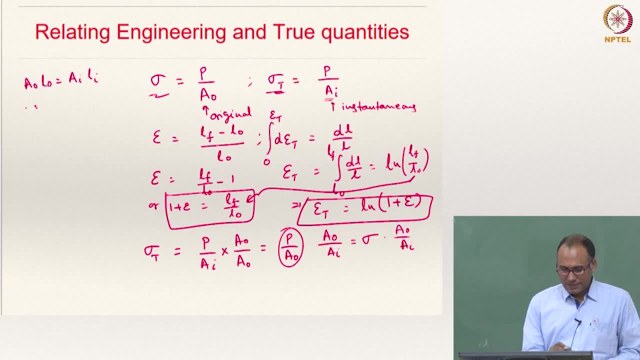 Is that acceptable? A0 divided by Ai will be equal to Li by L0.. Let us say this: Ai Li that we are talking about is Lf. that means the final length. all right, So then I can write this guy here. 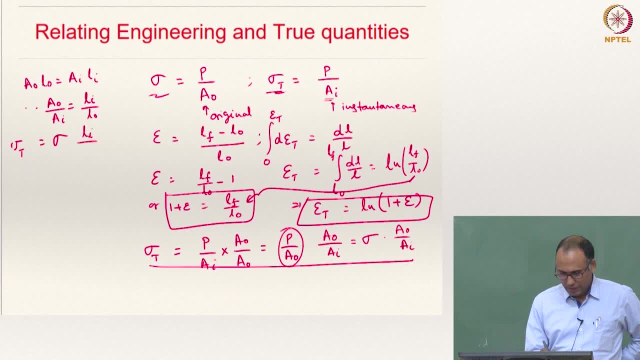 sigma T, equal to sigma times, Li by L0 or Lf by L0, the instantaneous one, wherever you want to find out. So what do I know about Lf by L0?? Again, I know that Lf by L0 is 1 plus, So that is how you can relate the true stress. 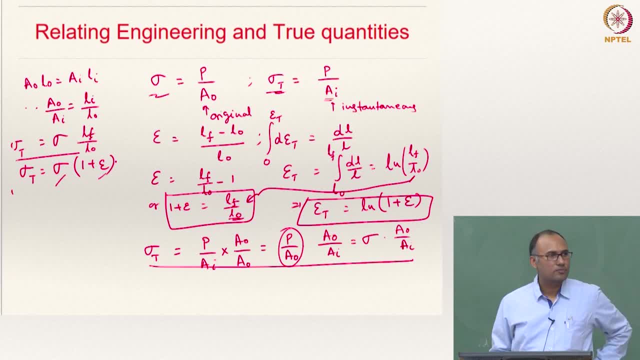 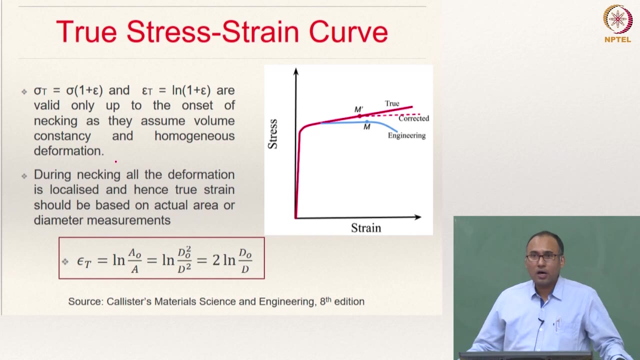 with the engineering stress and engineering strain, right? So, given your true quantities, you should be able to find out engineering quantities and vice versa, all right. So if you draw now the true stress strain curve, normally you would have drawn, you would have. 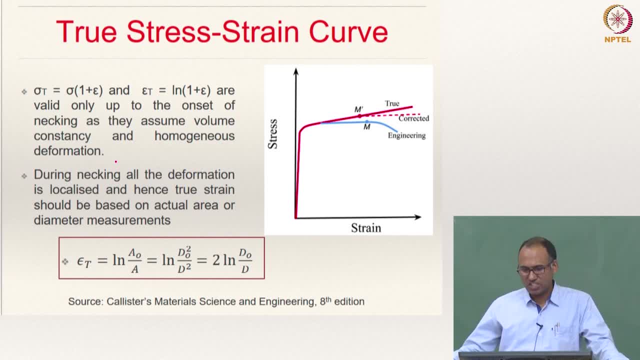 obtained out of your experiment. typically the engineering stress strain curve. that looks something like this: the blue color, blue color one, is the engineering stress strain curve. But if you would draw the true stress strain curve, when you are drawing true stress strain curve, your area should be instantaneous area and the instantaneous area when you are 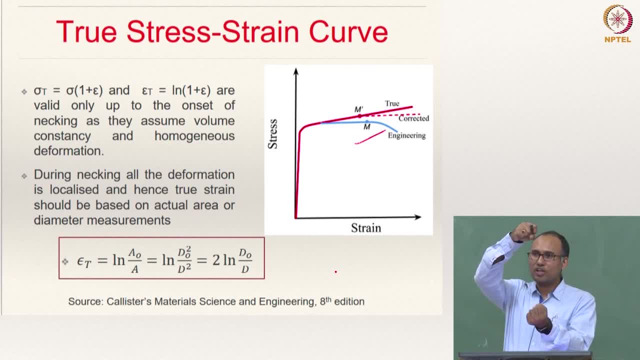 doing the tension test. Ai is going to be larger than A0 or smaller than A0. So you are going to be able to find out the true stress strain curve. Ai is going to be smaller because you are increasing the length. So transsection area. 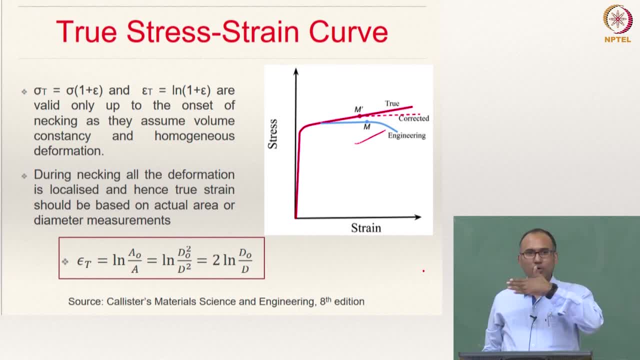 has to reduce. So naturally your sigma by Ai- sorry, P by Ai- will be having a higher value than P by A0.. That is why that curve is up. You can see that the red one is your true stress strain curve. 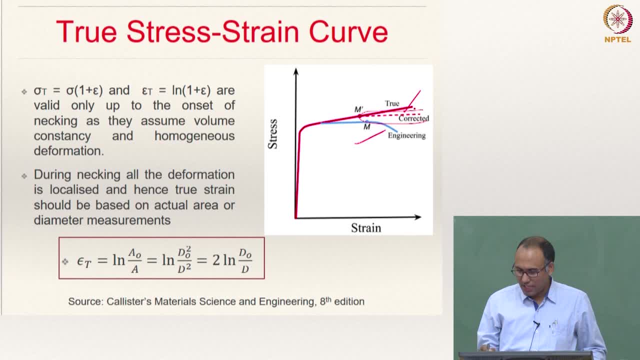 For the time being you will have the true stress strain curve, But for the time being you will have the true stress strain curve. So you will have the true stress strain curve. Forget about this dashed line. that is something called Bridgman correction. we will talk about. 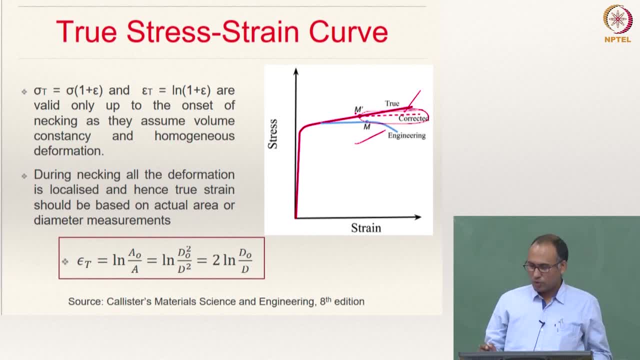 it in a moment, but for time being, do not think about it. you are only going to focus on the blue, solid blue line and solid red line. So the solid red line is your true stress strain And we have all just now derived, shown the relations between true stress and true engineering. 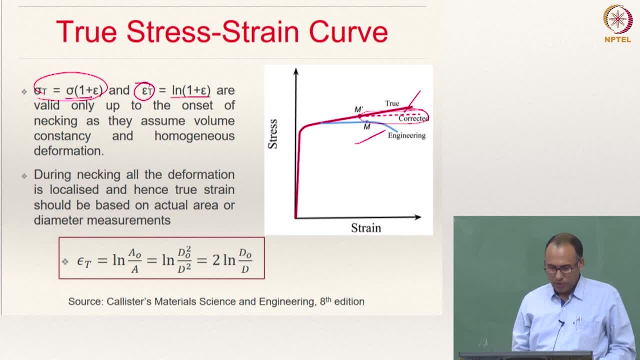 stress strain and true strain and engineering strain. So in the, when we have looked at our stress-strain curve, we have looked at this peak. that is what we call ultimate strength point. so the stress corresponding to that peak in the engineering 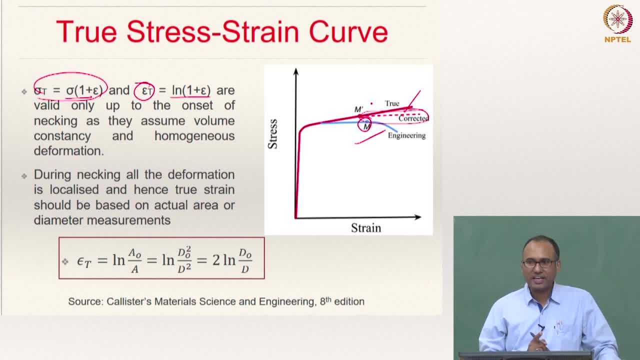 stress-strain curve is what is called ultimate strength of the material. So now, that is where in a ductile material- that is typically what is observed in a ductile material- The localized deformation takes place. that means, typically in a ductile material, this: phenomena called necking happens, So the local cross-section suddenly starts decreasing. this means all the deformation is localizing in that area. that is why it is called localized deformation- And eventually failure happens there. And that is the mechanisms. mechanism responsible for this. necking is in in ductile materials. 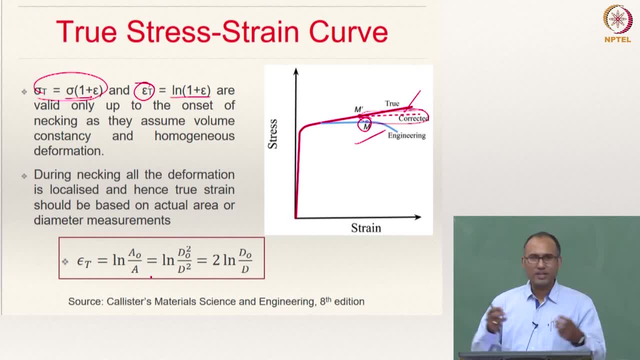 is actually void coalesced, Void coalescence and voids will coalesce with each other and, as a result, you will have net local reduction in volume. We have assumed volume constancy right until now, But then, the moment your necking starts, the volume constancy condition cannot hold good. 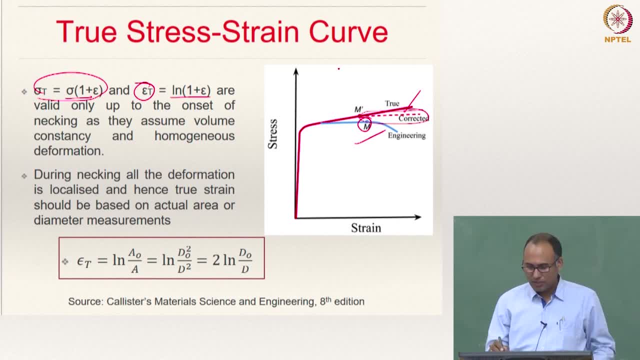 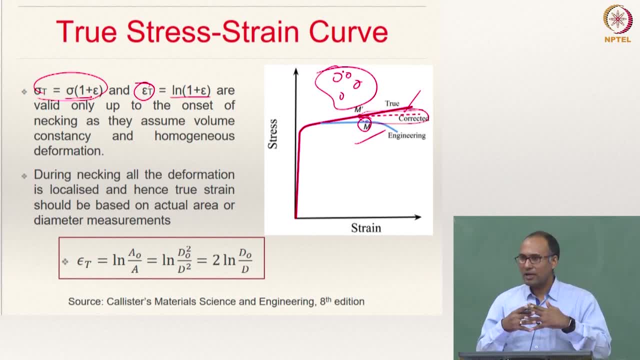 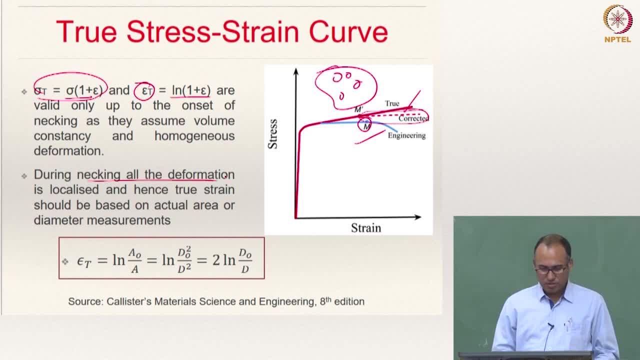 So during necking all the deformation is localized, So you cannot. if you think about the defining, for instance, true strain as a function of length, It becomes a little tricky because the deformation is localized and hence, instead of writing your strain in terms of lengths, you might want to write just before the onset of necking. 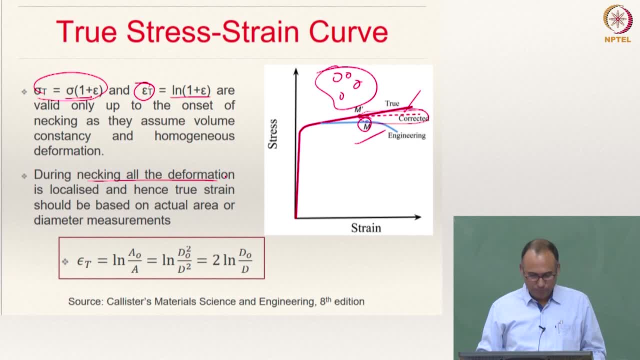 you might want to write in terms of area, cross sectional area, So you can use this. we have defined the relation between Ai just before the onset of necking. This is not during necking. just before the onset of necking, epsilon t will be ln A naught. 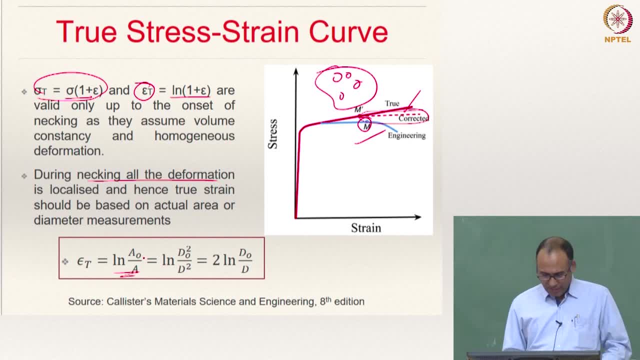 by A, And then you can write that as a function of d naught, assuming your specimen to be cylindrical. This is this expression is only true for a cylindrical specimen. If it is a some other specimen, then d naught by d does not work out because you have to. 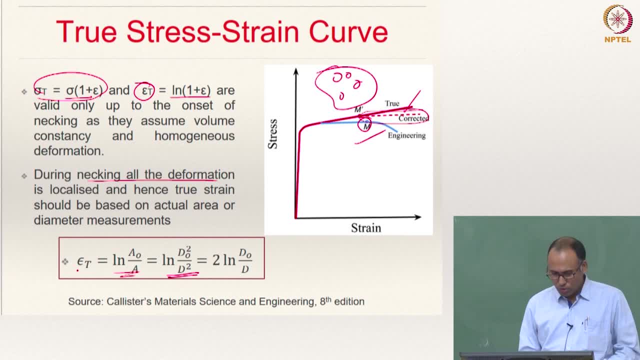 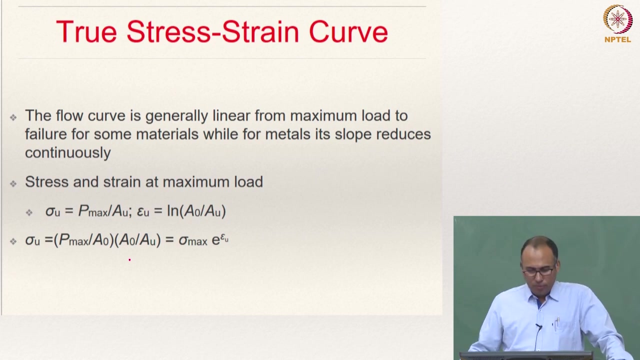 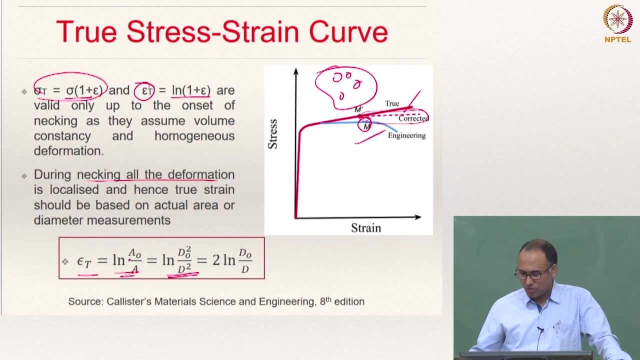 write appropriate cross sectional area for that. So the true strain in this case should be: usually is calculated using log A, So you will be. if it is a cylindrical specimen, you will be measuring the diameter in this process. So typically what happens is you have just now seen that your true stress strain curve. 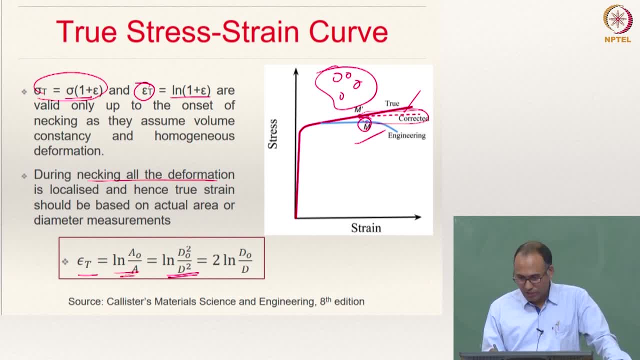 if you see, the corresponding point for ultimate strength point on engineering stress strain curve is m. On the true stress strain curve it is m dash And typically the true stress strain curve will always be left to engineering stress strain And then the flow curve beyond this point. it is many times it is found to be linear. 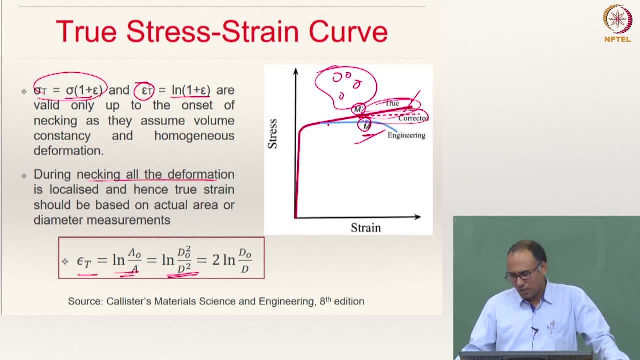 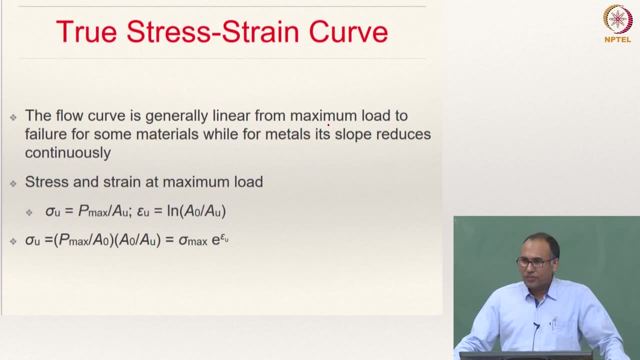 But sometimes it need not be, but many times it is found to be linear. For some materials it is linear, So it is linear, So it is linear, So it may be long linear too. And now, if you look at the stress, at the ultimate point, that means the where the 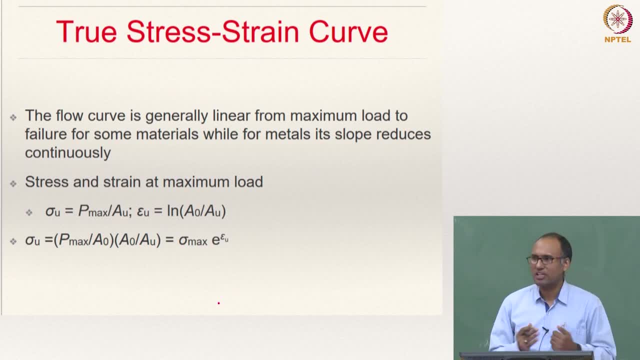 necking is happening. that is the maximum load carrying capacity of the material. It cannot hold any stress beyond that. After that actually a failure is happening. So that is why it is called ultimate strength of the material. So the ultimate stress sigma u is p max by a. 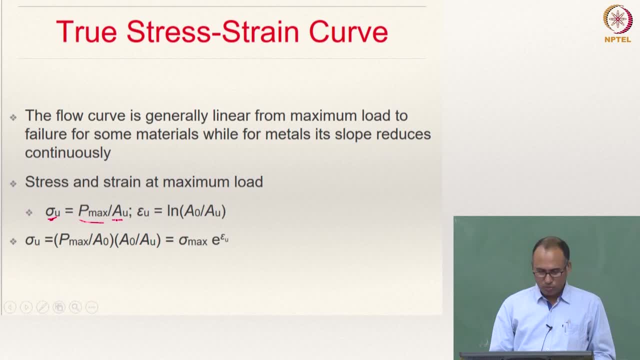 So you can calculate the ultimate stress at this point. So the ultimate stress sigma u is p max by a, And that means you can write this as to be a maximum load carrying capacity of the material. So Au is the area corresponding to the onset of necking. and then you can write epsilon. 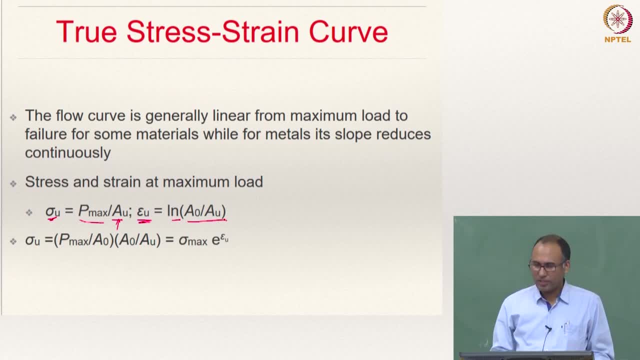 u, that is true. quantity is ln A0 by Au. that means corresponding to the onset of necking, that means the peak point. So you can write again sigma u in terms of P max and then connect that with epsilon u and see sigma max times e to the power epsilon. that is something that another relation particularly 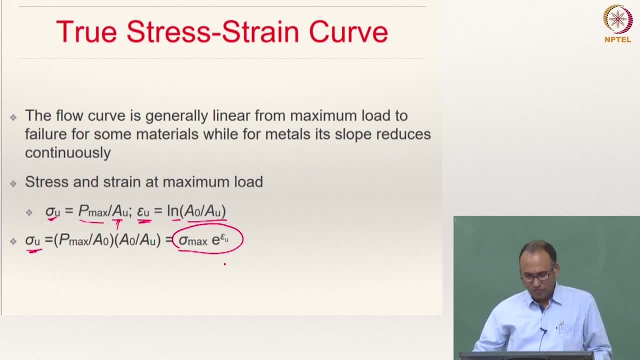 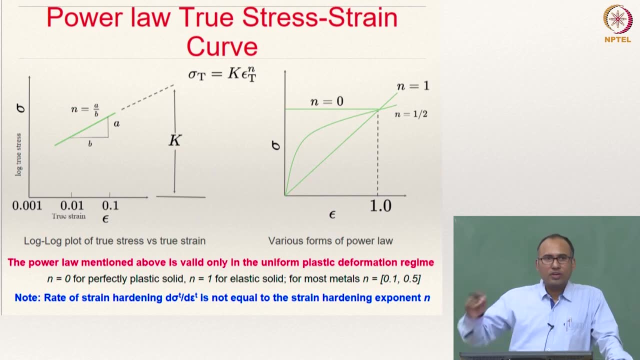 position where we are talking about the onset of necking Many materials. so we have the so far when we have done the uniaxial tension test. when we have looked at uniaxial tension test in the last class, we have identified the initial. 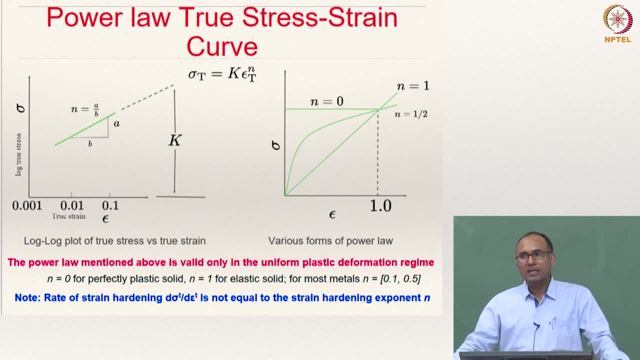 elastic region. That could be a linear elastic regime or a non-linear elastic regime. if it is a linear elastic regime, then the slope of the line in that linear elastic regime is called your elastic modulus. Slope of the stress-drive curve is what we call as elastic modulus or rank modulus of. 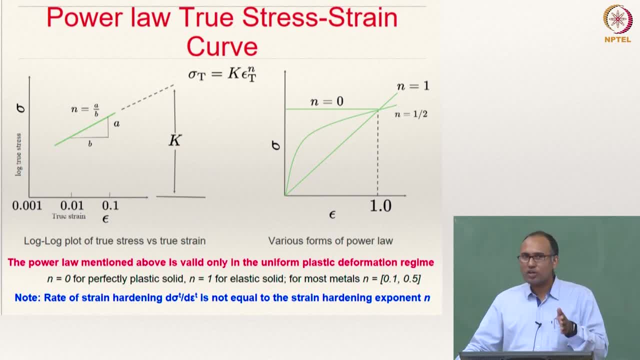 elasticity. If it is non-linear, this slope is not going to be constant, and hence you need to take something called tangent modulus. that means local slope, And that is what we have got. So we have learnt about the elastic regime, and then this elastic regime is followed by. 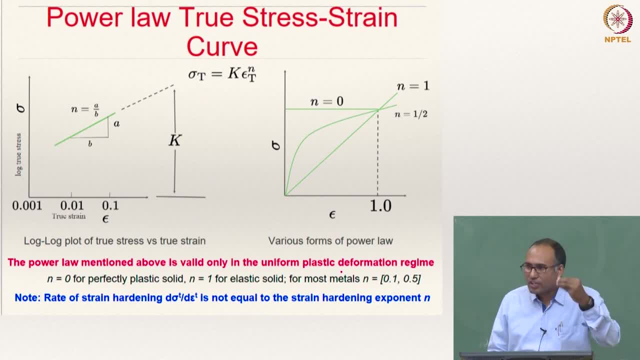 a phenomena called yielding. that means the onset of plastic deformation. That is when the dislocations in the material start moving. until then they are not activated. So that means your stress is not large enough to actually cause the dislocation. So at the onset of yielding. so that is why yield point represents the onset of plastic. 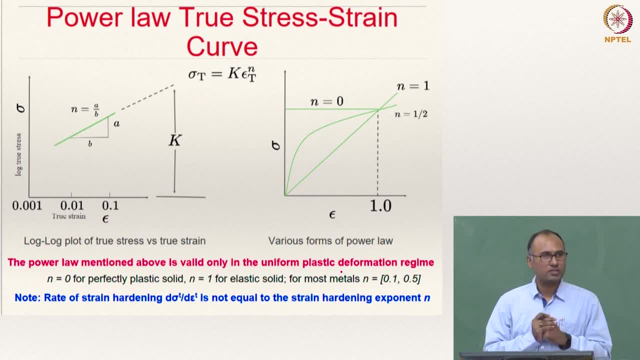 deformation. Until yield point you will not have plastic deformation. So that is again the property of the material right. Depending upon the kind of material that you are using, your yield strength will change. Similarly, your elastic modulus will change from material to material. 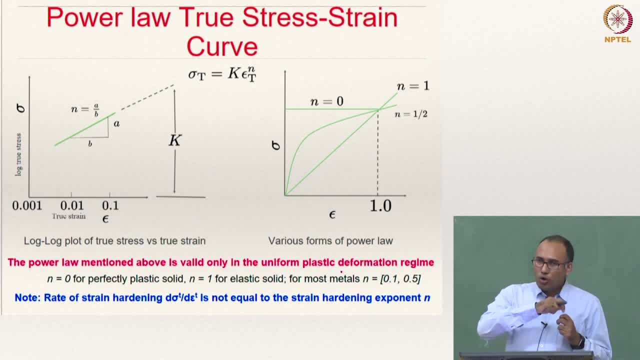 That is why these are material properties. And then, if you load the material beyond the yield point, you continue the plastic deformation, but the thing that you will observe is the material becomes hardened. That means it becomes harder and harder for you to cause further deformation. 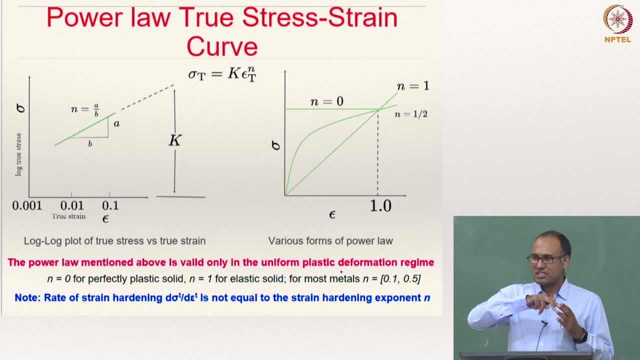 This is called a elastic deformation And this regime is called hardening regime. from the yield point up to the necking is called hardening regime And beyond necking. so once the necking represents the onset of localized deformation and then usually after necking, if you are looking at engineering stress-strain, curve your stress-strain. 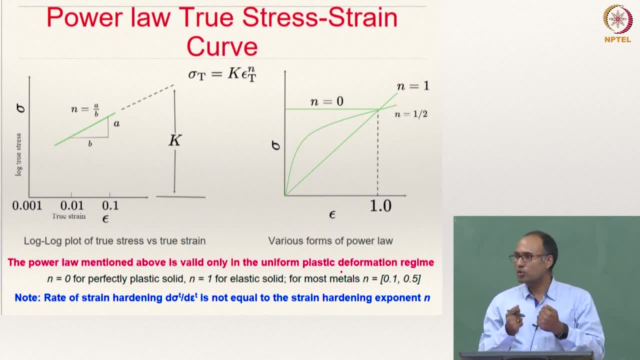 curve falls down because the force required to cause further deformation will go down Previously, until hardening until ultimate point, the additional force required to cause further deformation is increasing, was increasing, But after necking, the force required to cause further deformation goes down. 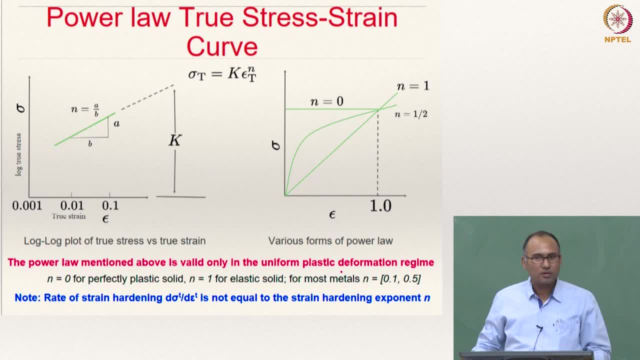 That is the reason why your engineering stress-strain curve goes down, because your P divided by A, So P divided by A goes down In the engineering stress-strain curve. the area is original cross-sectional area, which does not change, but P does change. 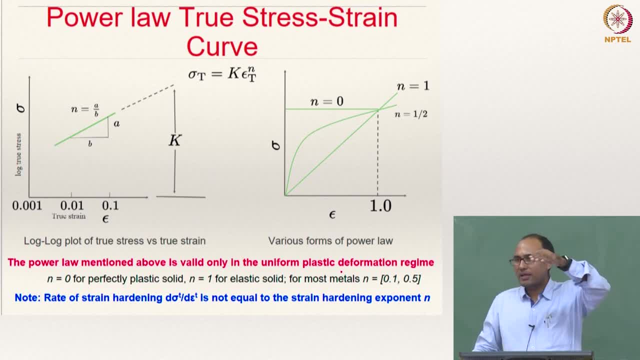 The fact that P is reducing. that is the reason why, beyond necking, the stress-strain curve drops. But engineering, if you take true stress-strain curve, why is it not dropping? it is continue to grow. that is because your cross-sectional area is actually reducing right significantly. 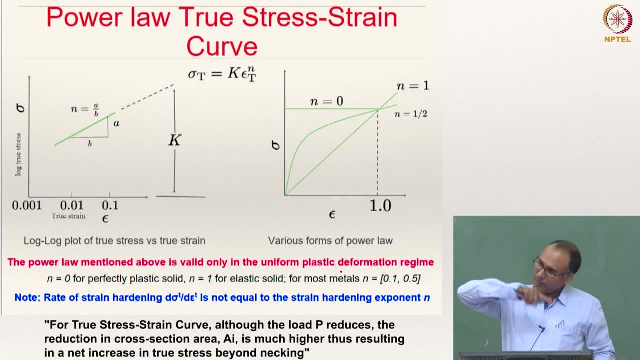 as you continue the load. So, although your requirement for P is increasing, P is also increasing, A is reducing, the total quantity is increasing, right? So that continues to go up. All right. Now we have defined the first region, which is called linear elastic rating. 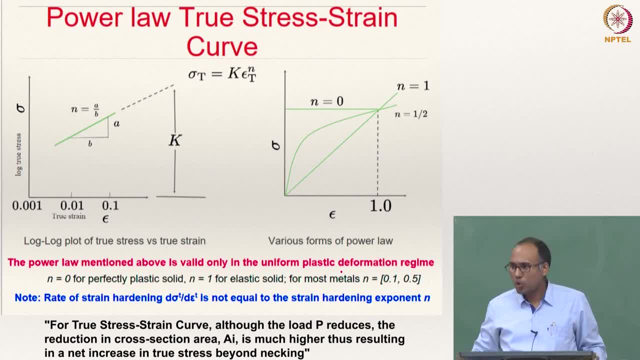 So we have a formula for that that is represented by Hooke's law right, Robert Hooke it is named after. Robert Hooke is English engineer or physicist who I understood the elastic deformation of the materials, who did seminal experiments in understanding. 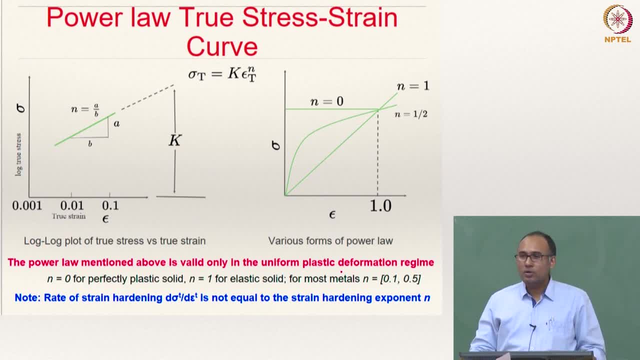 the mechanical behavior of the material right. So So sigma equal to E times epsilon is the formula that we use to represent the linear, elastic part of the system. And then how do we go about representing the hardening part? That means from the yield point to the necking. what is the functional form that we use? right? 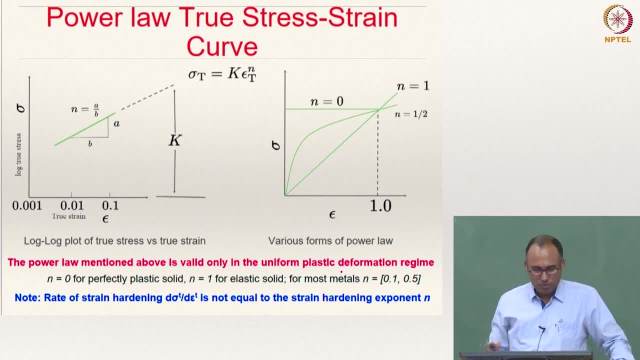 So there are several functional forms that are available. So usually the power law- true stress-strain curve. power law is one of the popular models wherein if you are plotting on the y-axis it should be like this: Right, It should have been sigma t because true stress-strain and true stress and true strain. 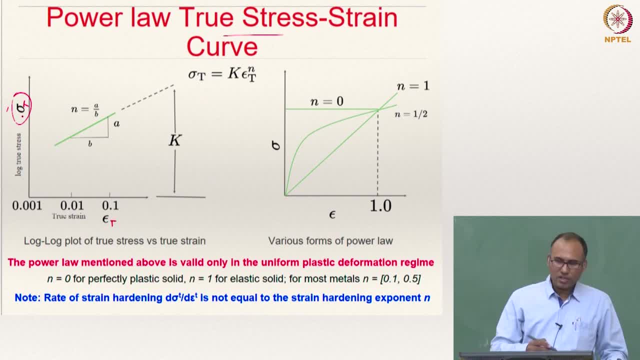 Then if you plot on a logarithmic scale, you will have a straight line, or in normal scale it will be looking something like this: And please note that this power law is a linear elastic Right. It is a linear elastic Right. 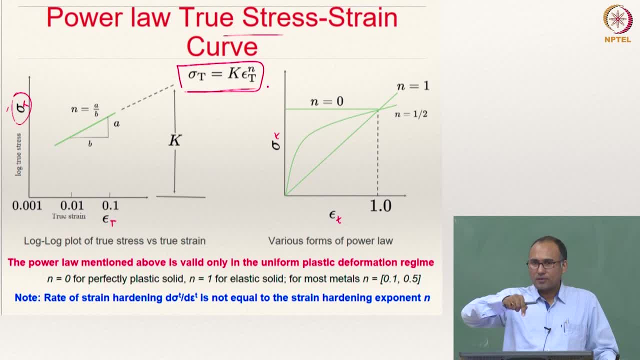 So it is from the yield point, not in the linear elastic. In the linear elastic regime it is. anyway, it is E times epsilon. ok, So there are two constants to represent the behavior of the curve. So this: if it is a linear n equal to 1, then it is called linear hardening. 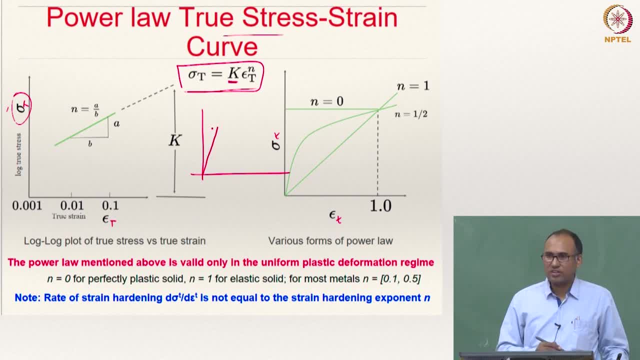 So you will have a material. This is a linear, elastic regime. So let us say: this is your yield strength. sigma y: From here onwards, the behavior you can have, no hardening at all. When n equal to 0, then sigma t equal to k, some constant, that is basically your sigma. 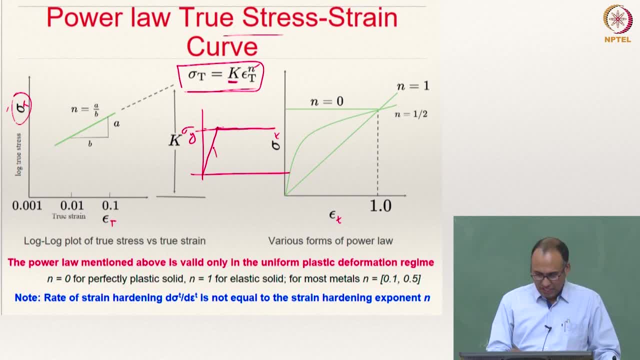 y, And this is what is called elastic. this is elastic, perfectly plastic material. There is no hardening at all. The material continues to deform at constant. That means, if you want to, if you were to see that from the microstructural mechanism. 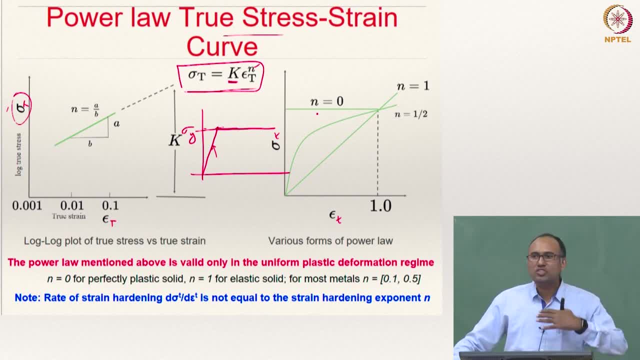 perspective, there was no resistance to dislocation muscle whatsoever And hence you are continue. you are able to. at the constant stress, you are able to have deformation. That means you are able to impart strain to the material. This is an idealization. 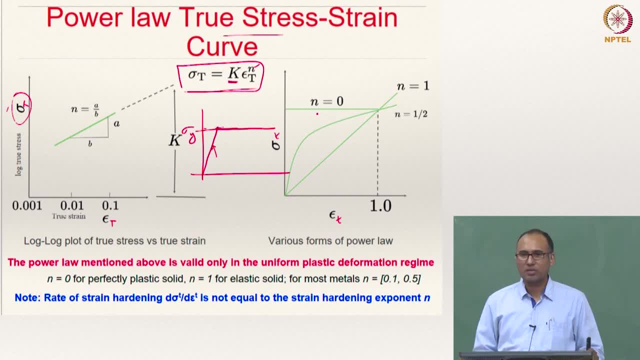 Typically, there are no materials which can actually show such a behavior, but it is an idealization. This is what is called elastic, perfectly plastic material. This is what is called elastic, perfectly plastic material. So several times, when you want to test the behavior of the materials in the plastic, 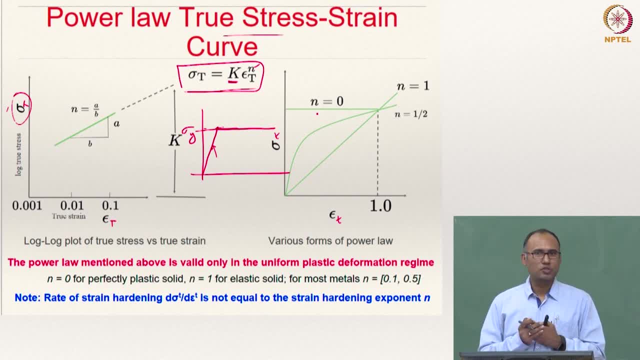 regime when you are writing your own numerical codes. the simplest possible thing is to do this, So you study what is the behavior of the system when the material is elastic, perfectly plastic, Because you do not have to worry about hardening, because you do not know much about the hardening. 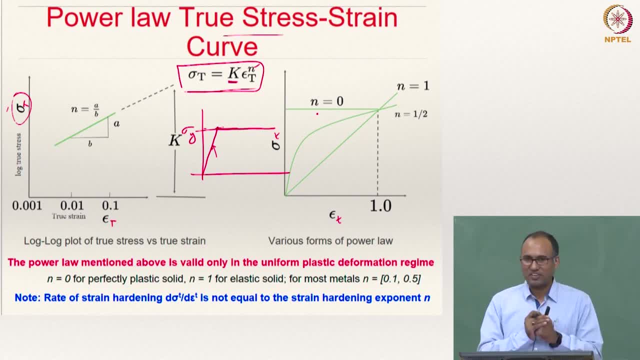 behavior. So, and hence you try what happens, if at all, it is perfectly plastic, which is an idealization, Which is an ideal case. And then, when n equal to 1, then this can be something like that, And this is what is called linear hardening. 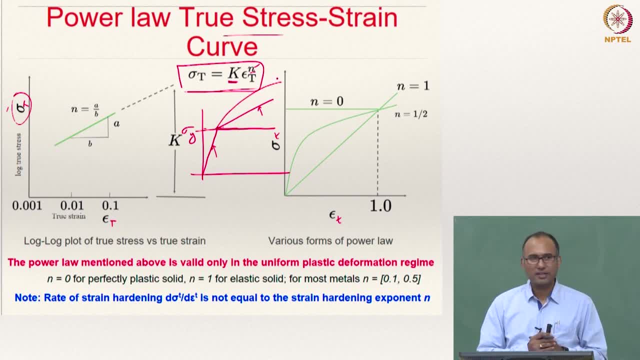 And you can also have non-linear hardening, something like that. So, depending upon the value of the exponent, you will have different responses. When n equal to 0, it is perfectly plastic. n equal to 1, it is linearly hardening material. 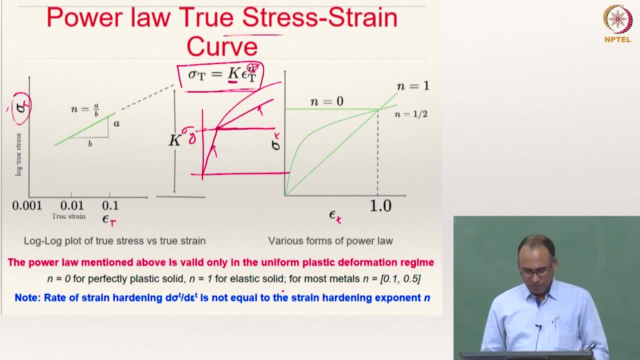 n equal to half, then it is non-linearly hardening material. Alright. So this power law is only valid in the uniform plastic deformation regime. So until the onset of necking there was no localization. The plastic deformation was uniform everywhere within the system. 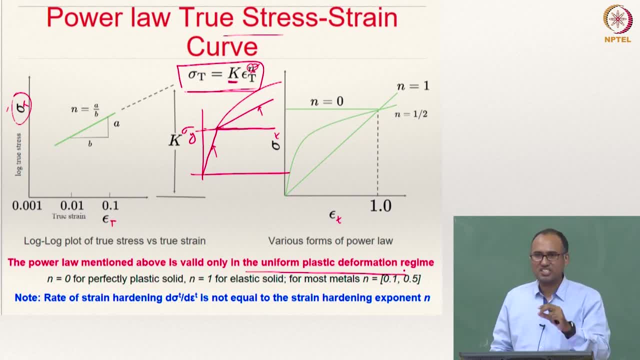 But the moment necking starts, the localization kicks in. That means you cannot call that situation as non-linear. So that is the problem. So this is the problem. So this is the problem. How do you call that situation? 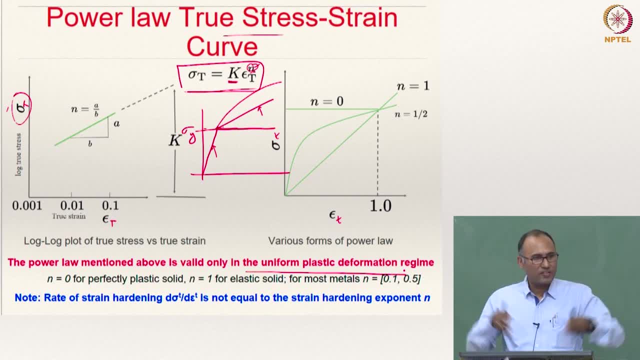 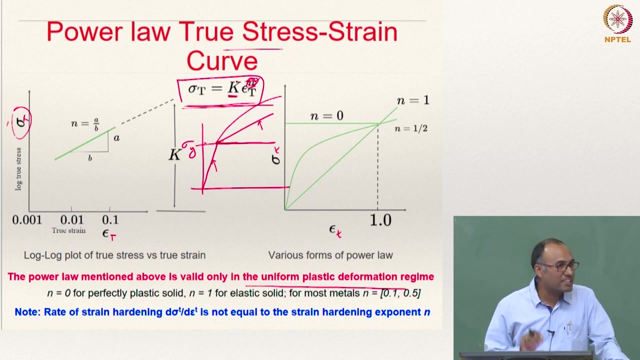 Uniform plastic deformation. All your plastic deformation is happening at one place. Everything else is sitting doing nothing. So this power law formulation is only applicable until as long as your material undergoes uniform plastic deformation. This n is what is called train hardening exponent. 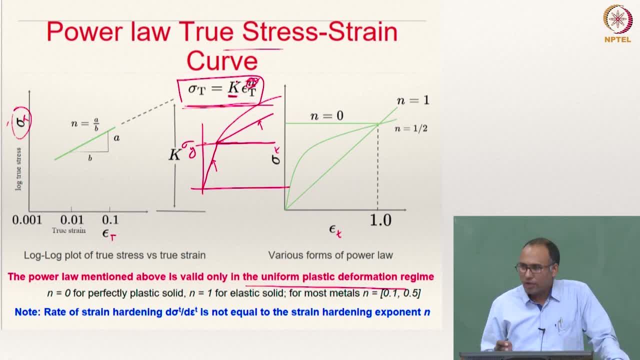 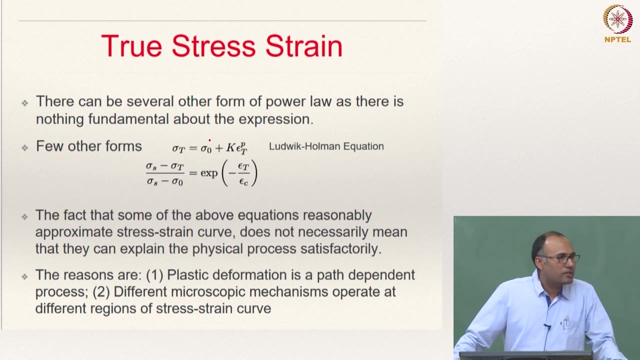 It is a material property again, Depending upon the kind of the material, Whether you have a linear or a non-linear nature. Okay, hardening or non-linear hardening and so on. So this n is what is called strain hardening experiment, And we have given one form that sigma t is equal to k times epsilon t power. 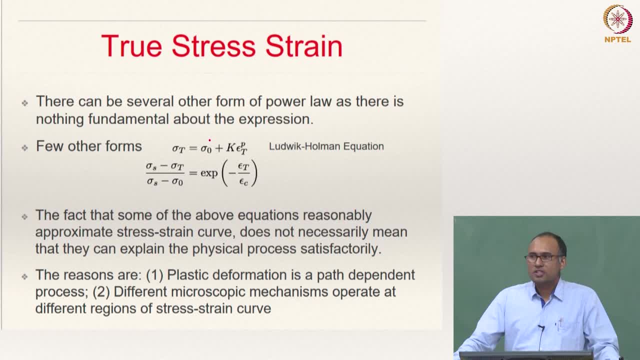 n. But there is nothing special about this form There is in principle. you can write different kinds of forms that you want. People can come with different kinds of forms as long as they match with the experimental rules. So that is why I am saying there can be several. 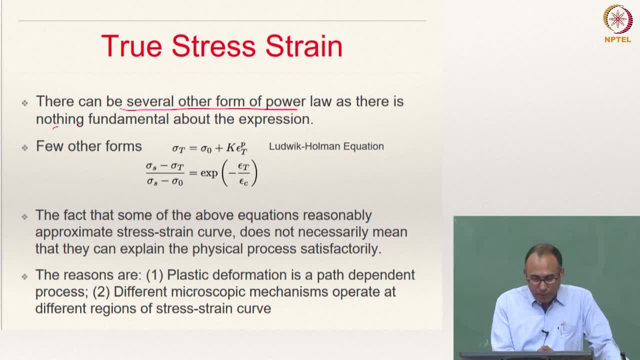 other forms of power law and there is nothing fundamental about the expression. So you do not have to have so much of attachment to this power law, the way that we have written. There are other forms. for instance, this is another form which will say that you can: 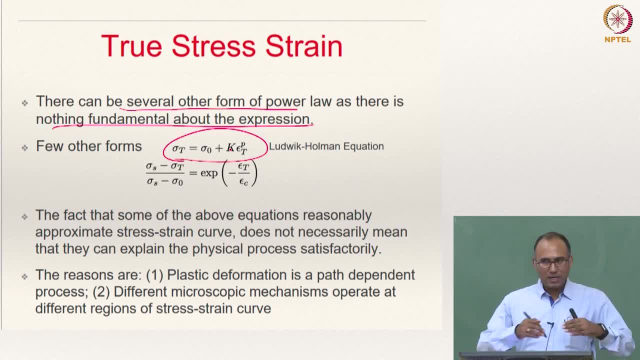 write that it will include your plastic strain. you have written in terms of plastic strain because until elastic regime- it is, plastic strain is 0. So you have taken that into account and then you have written that without actually worrying about where you are starting. 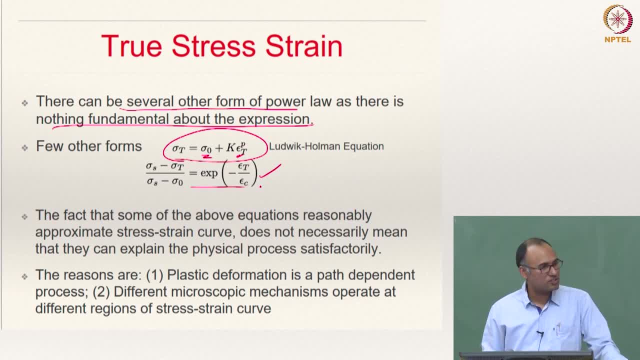 this, And there is another expression which is an exponential form, written this: So all these forms are possible, And also some of these forms. so people come up with different forms. So you have to come up with different forms of this expression because somebody has given. 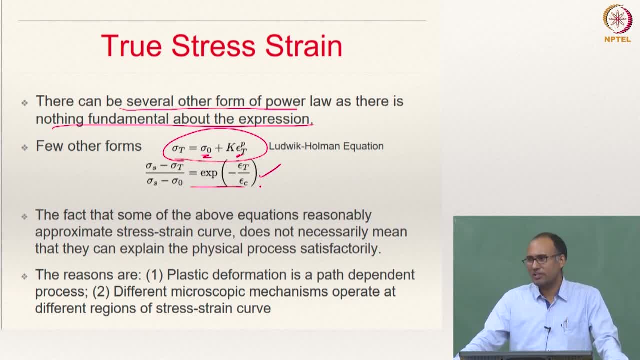 power law and they have done this experiment, their experiment for the particular material, and this set of materials does not seem to follow the power law. Then they have looked at it. the power law is not working. So this is not a power law material, but it is some. 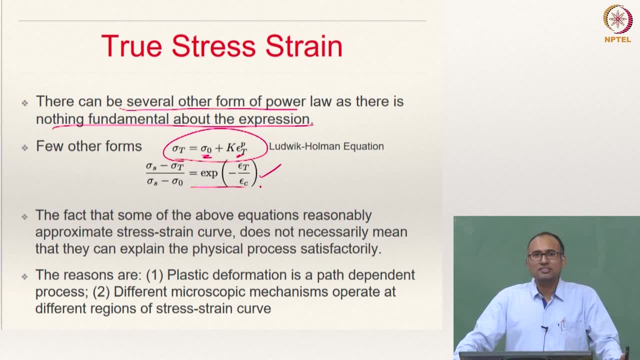 other material. So material is behaving the way that it wants. It is just us who are associating some mathematical form to it, So, and hence we should not. So you have to come up with different forms of this expression, because somebody has given. 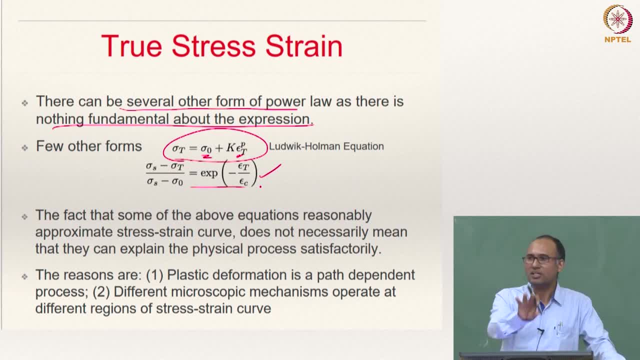 you some material, So this is why we are asking you to come up with different forms Now. we have attached too much of value to the particular mathematical form that we are attaching to this behaviour, and no matter what mathematical form that you attach it. 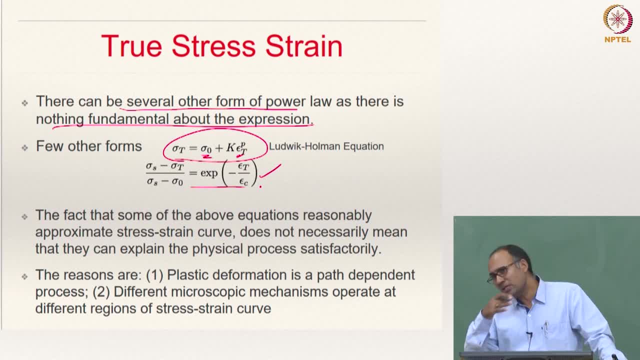 may actually match very well with the experimental results, But that does not mean that it can actually explain all the mechanisms- microscopic mechanisms, at play in the medium. You are just hypothesising the macroscopic behaviour of the material, So you write that it is. 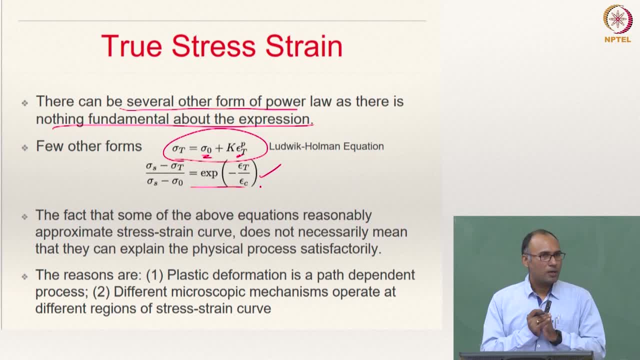 but you do not write that it is a material, So you have to come up with different forms: material through a mathematical form, But that in most way can represent all the microscopic mechanism, because it is all. after all, this is a law describing the macroscopic phenomena where you do not have any information. 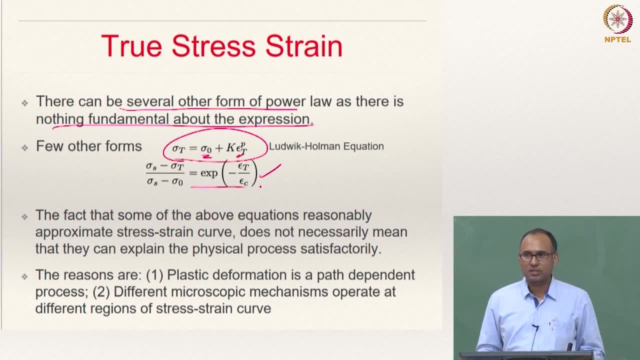 about the microscopic deformation mechanism right, And hence we should be very much careful when we are looking at these stress strain relations in the plastic regime, particularly because there can be several other forms one can fit in And that form can work for a particular class of materials. the same form cannot possibly. 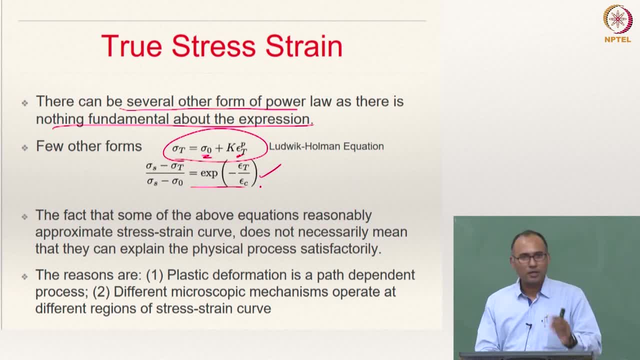 work for other class of materials. so you please keep that my that thing in your mind. And the reason why sometimes it may work and sometimes it may not work is because, primarily, the plastic deformation is a path dependent process. That is a very important thing to remember. so because when you are writing your, for instance, 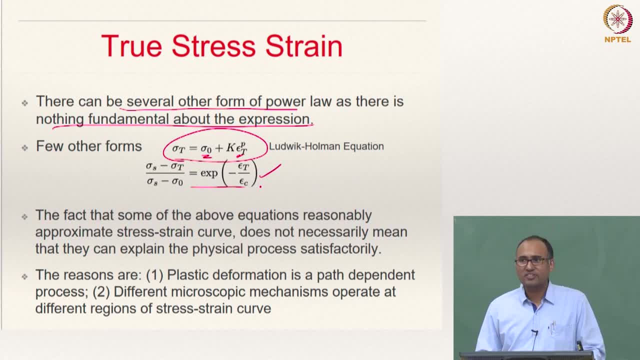 if you are modeling plastic deformation in a material, it is extremely important that you actually carefully follow the path dependence. Otherwise you will be actually estimating your stress state in a completely wrong manner than what it is supposed to be. okay, And of course, we have discussed that there are different microscopic mechanisms. 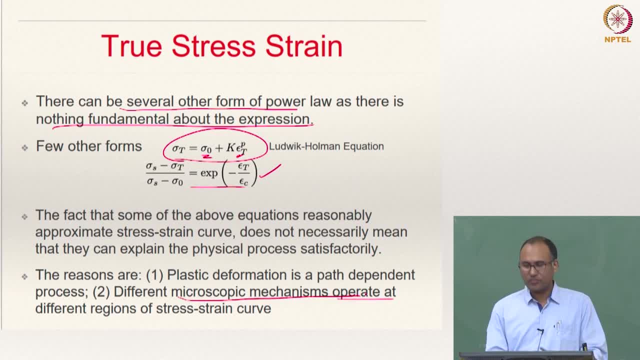 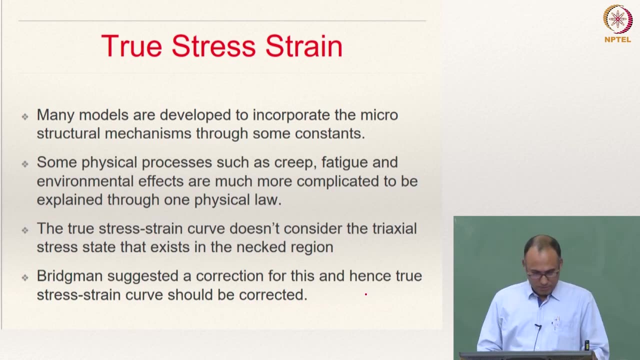 Okay, That can be operating at different regions of the stress strain, So you possibly cannot use one law to describe every part of the stress strain. alright, So, as we have discussed, there are many models which are developed to incorporate the microstructural mechanisms through some constants like the k and n. 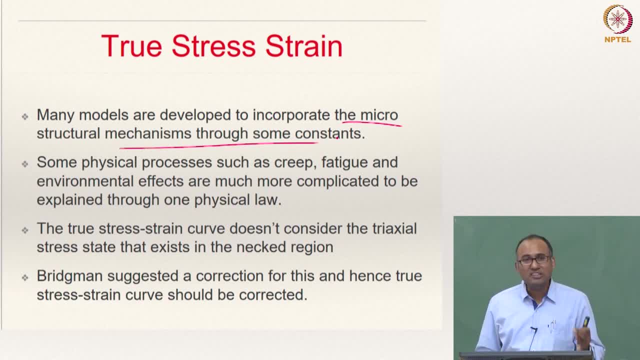 These constants sort of represent the microscopic mechanism in some average sense, but they cannot represent the microscopic mechanism at each and every point on the stress strain curve because the mechanisms themselves might change when you go from one region to other region. For instance, some physical processes like creep, fatigue and environmental degradation. 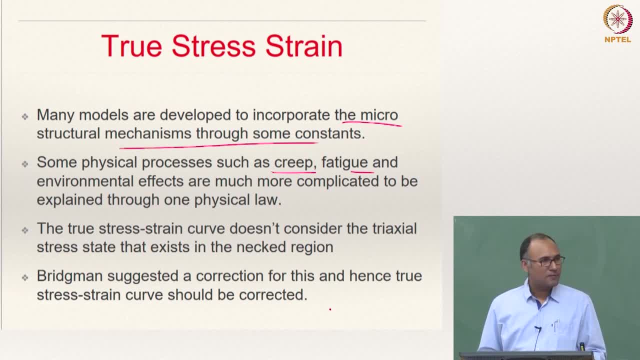 such as corrosion, are much more complicated to be explained through simple laws that we have discussed. Okay, So it is simply not possible. So if you want to incorporate new mechanisms, you probably have to deal with more and more complex models to describe the mechanism. okay, 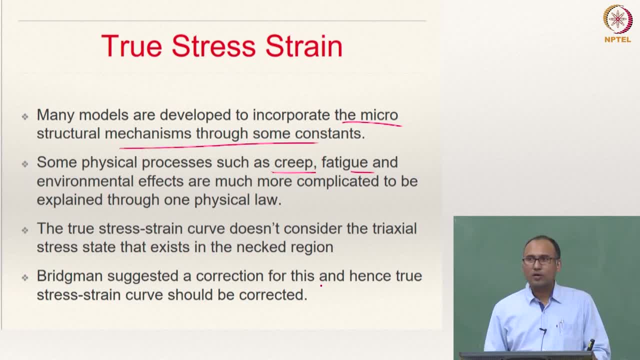 And, as we have discussed, it is not going to take into account the true stress strain curve, does not consider the triaxial stress state that exists in the neck injury, So it does not worry about the true stress strain curve, does not take into account of 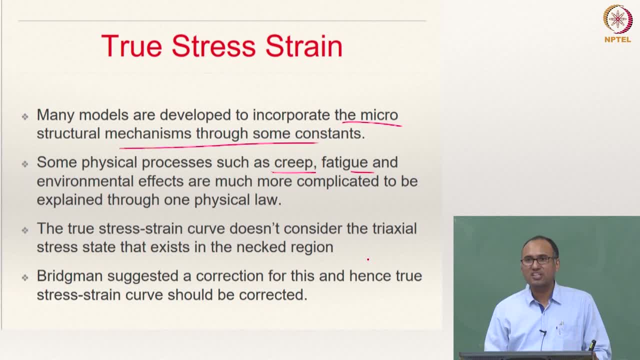 this triaxial stress state. Okay, So it is not going to consider the triaxial stress state that is existing in the neck injury And, as a result, that means there is local hydrostatic stress that is present during neck injury And that is not usually taken into consideration when you have drawn the true stress strain. 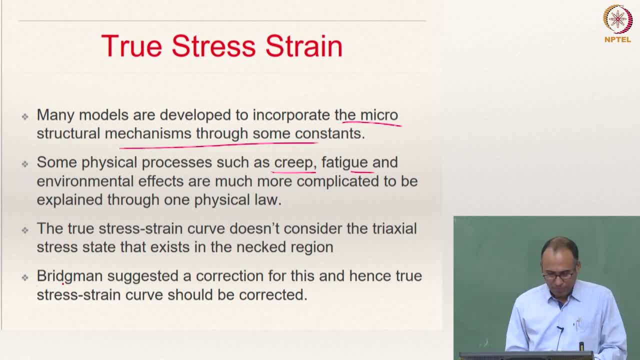 curve, but which has to be considered. So Bridgman did some experiments And he suggested that you need to take into consideration of the existence of the local hydrostatic stress state of stress during neck injury. We will talk about it when we are done. 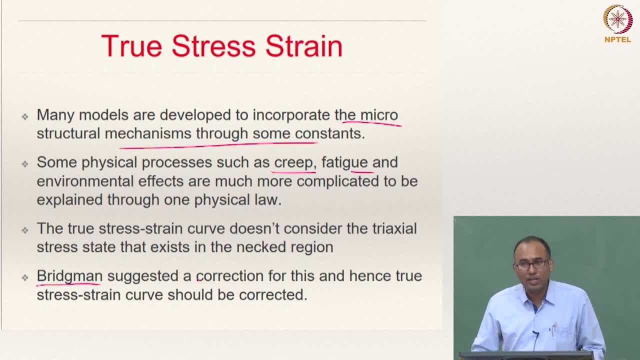 We will talk about it when we are going to discuss failure theories- why one should be concerned about local hydrostatic stress in this situation. So he suggested- and hence the true stress-strain curve, the way that it is drawn, the solid red line is not entirely true. 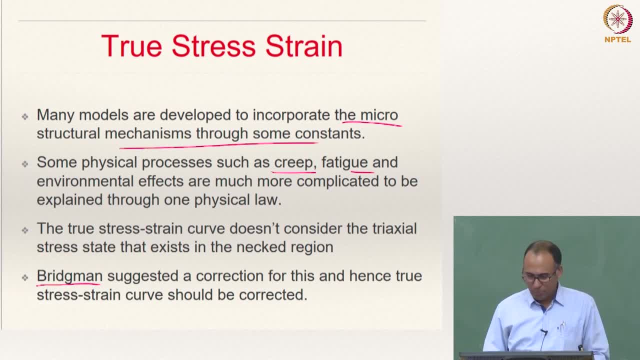 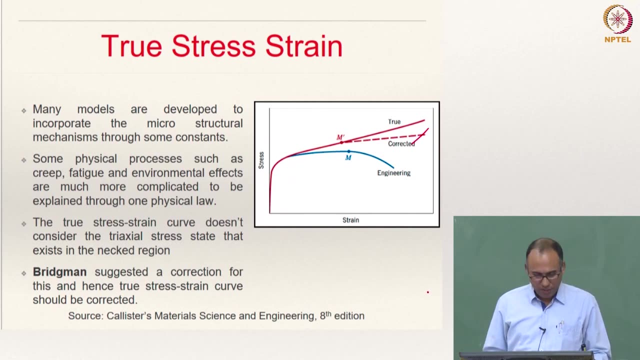 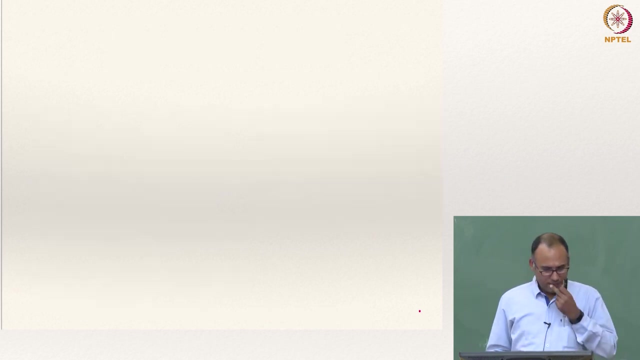 You need to account for some correction, which is which has been suggested by Bridgman, and hence the dashed line came in. That is the true-true stress-strain curve. yeah, all right, so this is the corrected. the dashed one is the corrected stress-strain curve. all right, so I think I have. I wanted. 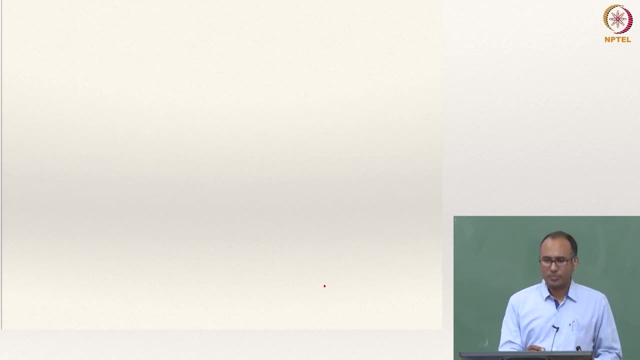 to also discuss with you another concept before going on to. okay, let me finish this conditional definition for onset of necking right? so when you are drawing engineering stress-strain curve, so that is your ultimate tensile strength, so that is the onset of necking, right this? 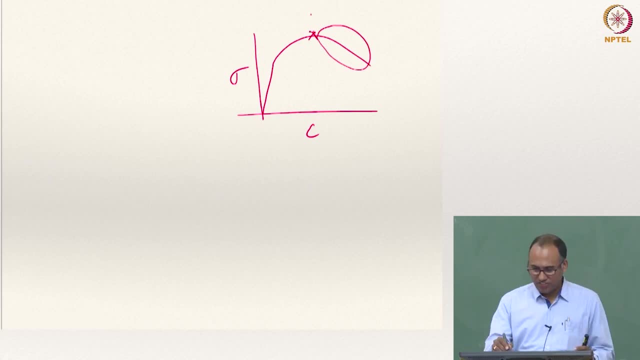 is the process during which necking evolves, but the onset happens here. Necking is not progressing, here, it is just started. it is like this point where flashed started, it did not progress. similarly, necking started, it did not progress. this is where 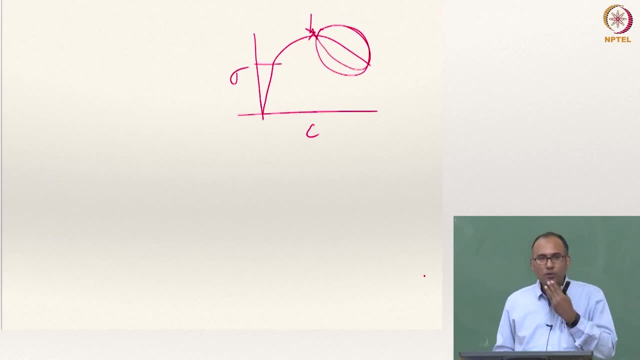 the necking is progressing. okay, now you can actually write from the load perspective. you can write this as dp equal to 3, right variation. that is a peak point, right? so you can write p equal to sigma t times a. is that acceptable? 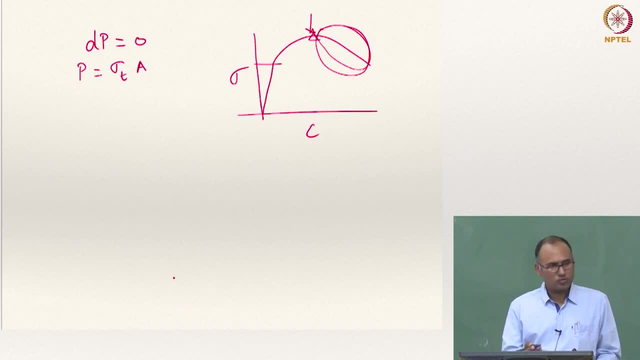 Yes, Okay, Yeah, that is what we have learnt, so I can write the variation of p as sigma t. da plus d, sigma ta must be equal to 0,. right And now. I will leave you here and now, if our hardening response is represented by sigma. 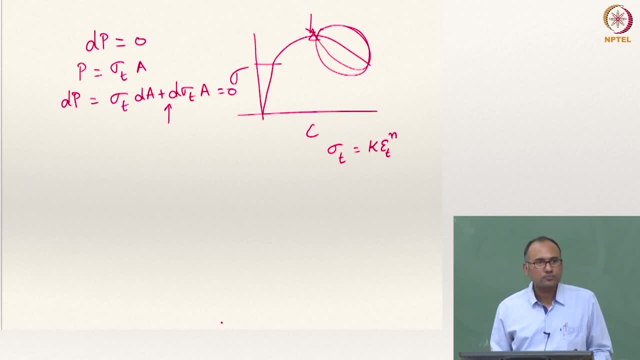 t is equal to k epsilon t power n. what is the condition for necking? what happens at the onset of necking to d sigma t by d epsilon? can you go about deriving that? So we start here and you know everything about the stress strain relations. 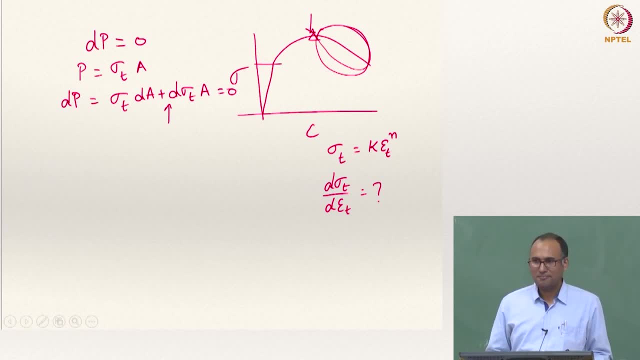 Okay, Okay, Okay. So now I want you to find out this line, so you know that at the onset of necking, this is the condition, so you can clearly see that d sigma t by d epsilon t is equal to k n epsilon t power n minus 2, right, but at the onset of necking, what happens to this? 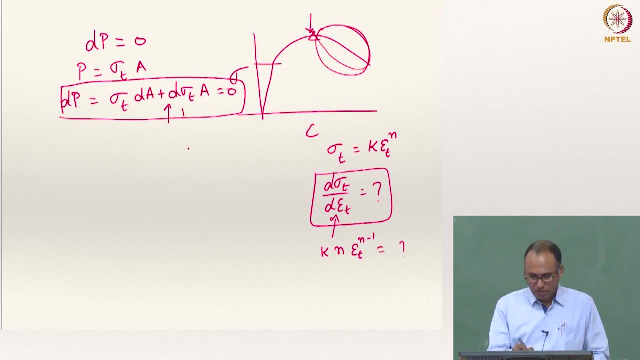 this must be equal to something. Okay, Okay, Okay, That should come from this. Can you find a relation between sigma t, d sigma? so what is normally? you say that if d sigma by d epsilon must be equal to 0 at the onset of necking right? so similarly. 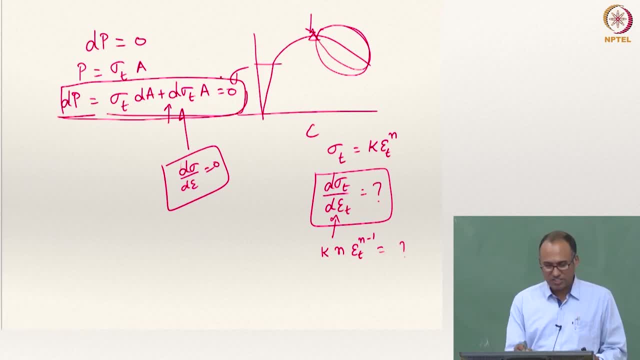 d sigma t by d epsilon t. that is actually equivalent to this k right, this condition is same. So now you have a variation in area. so you can write from the volume constancy da by a in terms of bl by l. 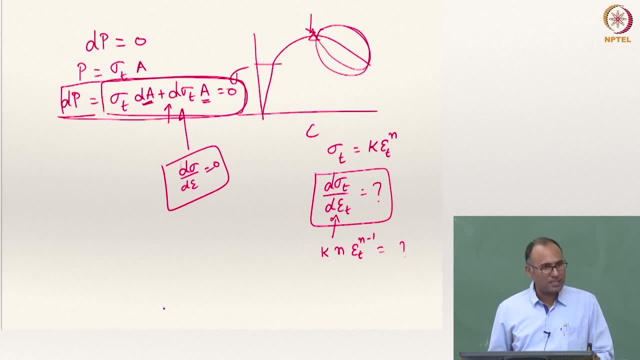 Okay, Okay, Okay, And from there you can bring in the true stress strain value, right, and hence you would be able to correlate d sigma t by d. you can get d sigma t by d epsilon t from here. what should that be equal to? and then equate that to this guy? so you have to get what is d. 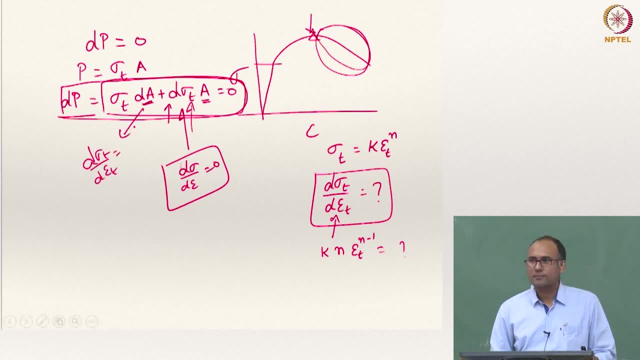 sigma t by d epsilon t from this relation, right, and that, equate that to this guy. and then you will say: Okay, Okay, Some something coming up. so at the necking d sigma t by d epsilon t is not equal to 0,. 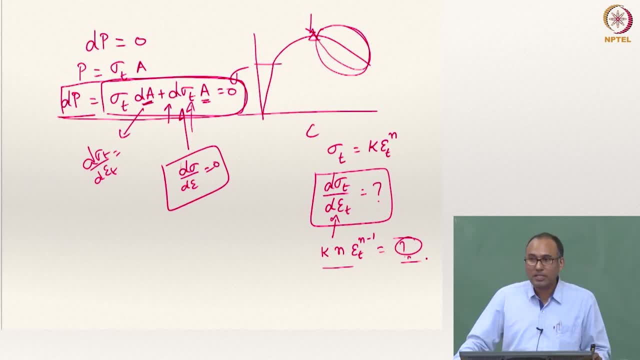 right, it is not equal to 0, d sigma t by d epsilon t is not equal to 0 because there is no peak in true stress strain curve. d sigma by d epsilon is equal to 0 or dp equal to 0. 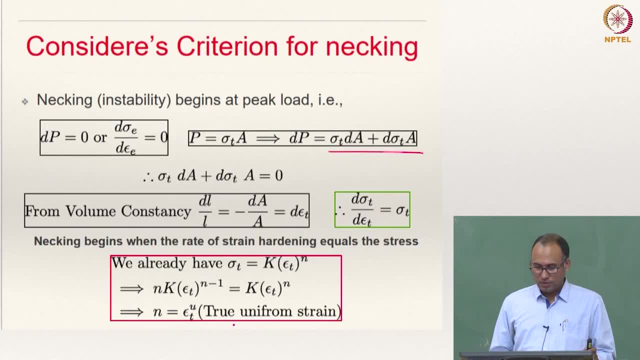 Okay, So this is what I have written right. So dp equal to 0. From volume constancy, dl by l, equal to minus da by a, that is d epsilon t. and then you can write d sigma t by d epsilon t is sigma t right, which means this is sigma t. 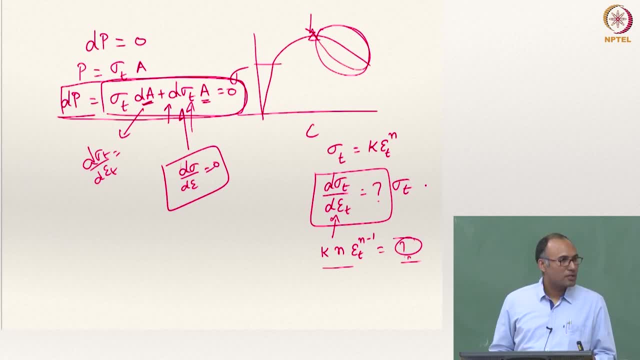 So the variation of true stress, the necking begins when the variation of true stress with respect to true strain becomes equal to true stress. That is when necking begins. Okay, That means again, if you want to further work on it, epsilon: t power n divided by epsilon. 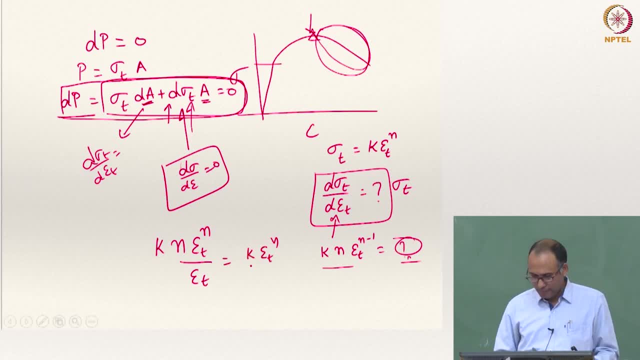 t is equal to sigma t minus k times epsilon t power n, k, k gets cancelled. epsilon t gets cancelled. Therefore epsilon t equal to. in other words, when your true strain becomes equal to n, the hardening exponent Okay. 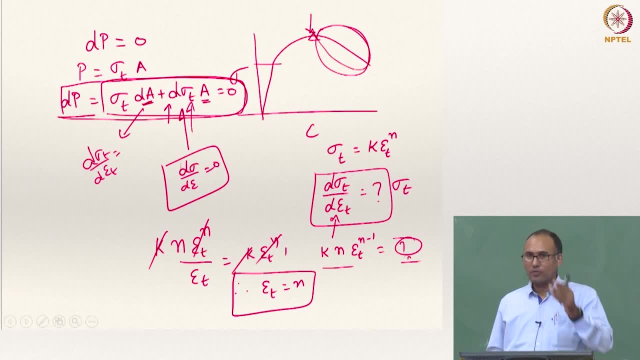 That is when the necking begins, Right. So in the case when you are writing from the perspective of true quantities, the necking begins when the rate strain rate of change of stress in true quantities becomes equal to true stress. That is the key d sigma t over d epsilon t becomes equal to epsilon. 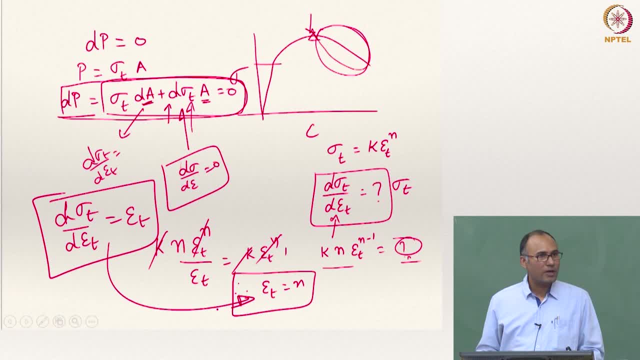 That is nothing but this. When your true strain, Right, That is epsilon t, u at the onset of necking, that is u I have written because it is ultimate point. Right, That must be equal to n. That is when necking begins. 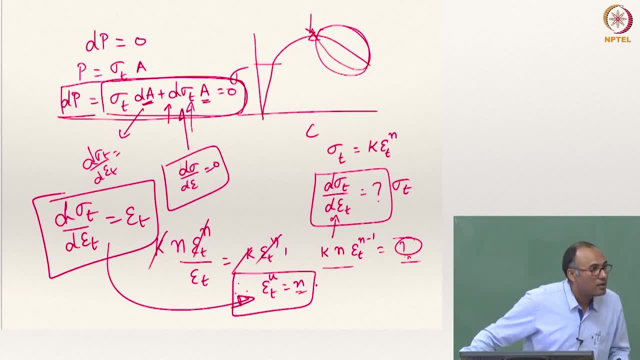 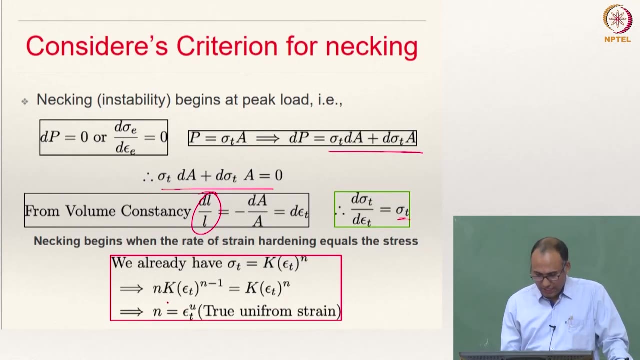 Oh yeah, Sorry, Sigma t, I have said sigma, but I have written epsilon. Thanks, Yeah, All right. So let us see, Let us see, Let us see, All right, So you can actually say that when n is equal to epsilon t, u? u is the ultimate at the ultimate. 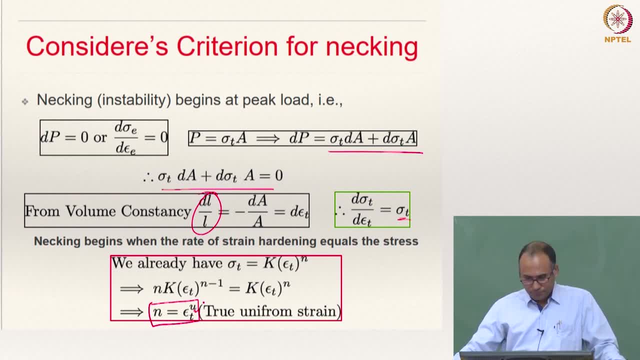 point, because that is where we are saying the necking begins. Okay, So this criterion for necking is called considerer's criterion, So considerer has given this criterion. in terms of true quantity, It is a name of a person. 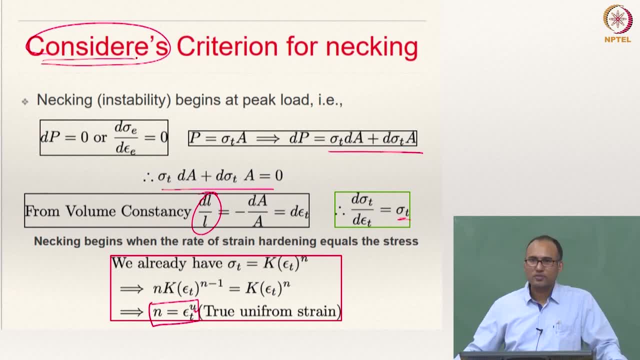 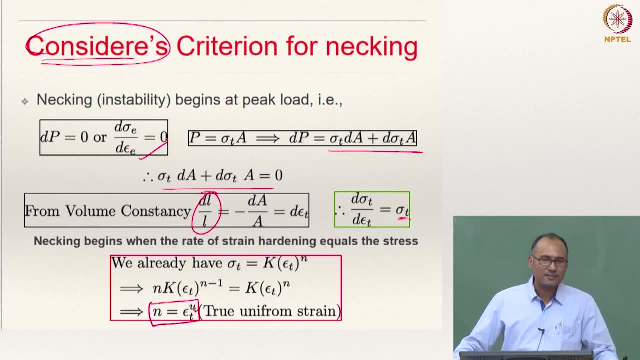 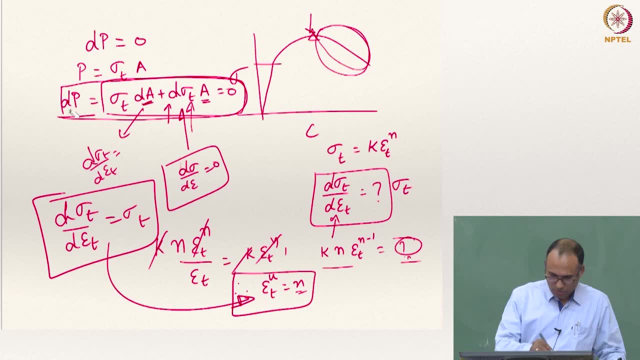 e by d, epsilon e equal to 0.. Yes, All right. So before I move on, I would like to spend couple of minutes on giving little bit more understanding. Let us say you have this stress triangle For time being, let us draw engineering stress triangle. 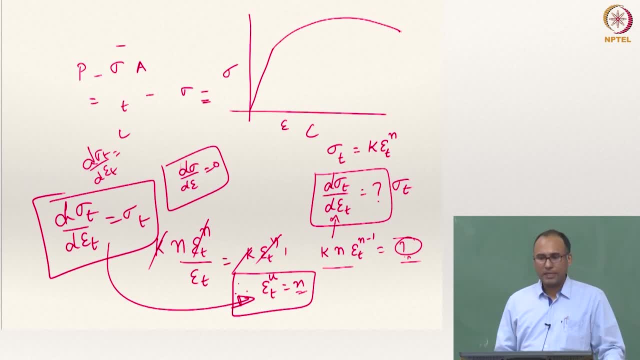 All right, Now I am doing this stress and this is my sigma y. Now let us say I have loaded this guy up to here, Okay, And then I decided to unload What happens. I have loaded up to this point. 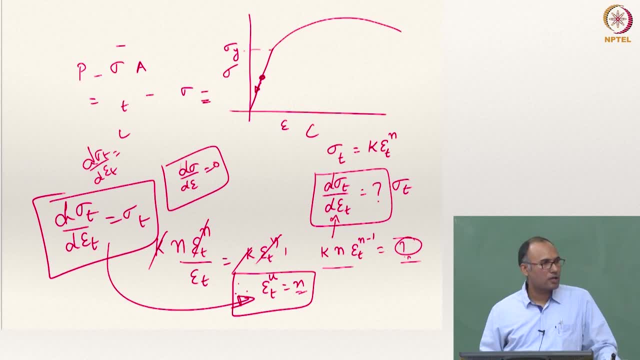 Now I decided to unload. I will come back around. Okay, So I will be able to come back here. So what is the amount of plastic strain at this point? 0.. There is no plastic deformation and hence it should be 0. 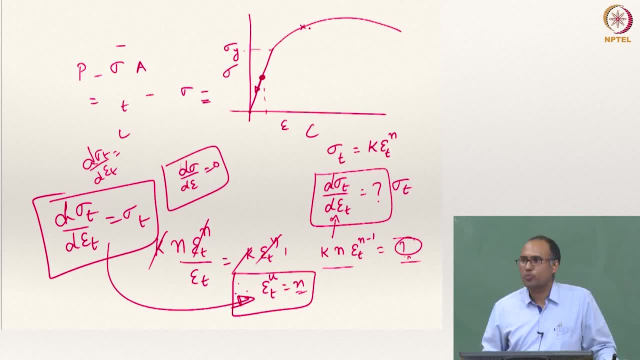 Now, let us say I have loaded up to this point. Okay, Now I have not gone to the region of necking, I have only loaded up to this point. And now, if I unload, what will happen? What will be the path? 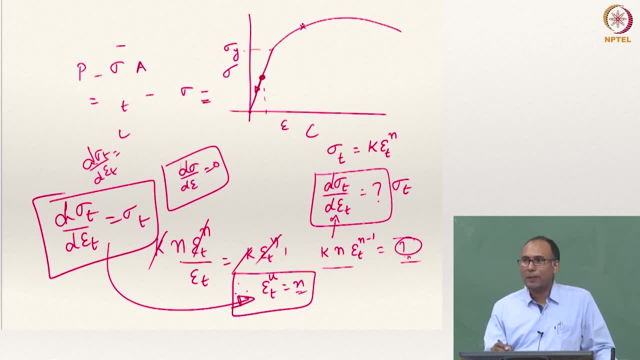 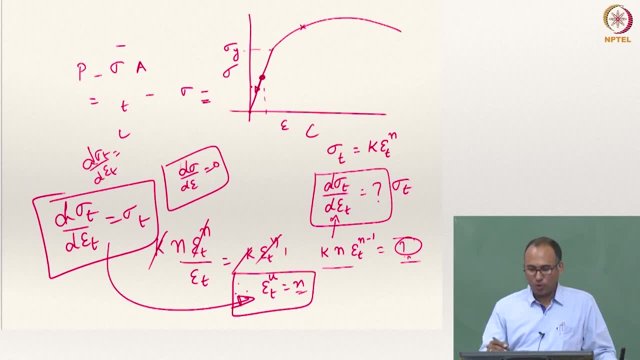 Parallel to 2. Parallel to This region, This line. Okay, What did you say? Poop's region? Okay, So you will unload along a line whose slope is equal to your elastic line. Why should it be parallel to that guy? why should it only unload along that line? 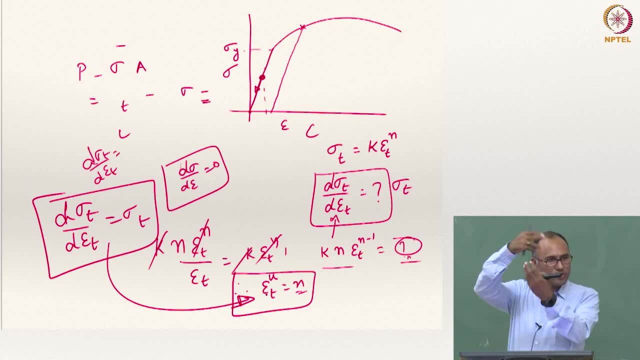 Because when you are unloading, you are not causing plastic deformation. your plastic deformation is over All. the unloading is only elastic, right. So elastic behavior is described by elastic stiffness. So that is the reason why it has to only go along that path. it cannot choose any other. 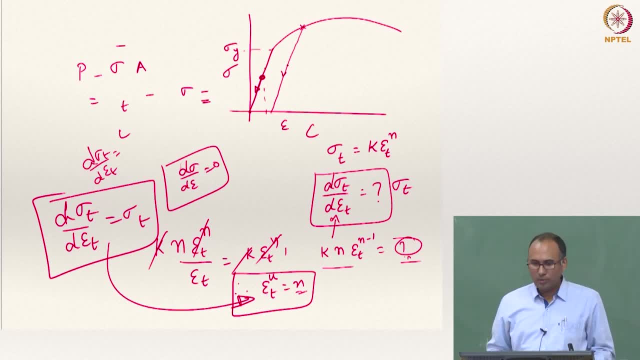 path. So this is your unloading path. very good, So now, when you have loaded the guy up to here, your total strain. you please pay attention here, it is very important concept. This is your total strain. So let us say 0,, A, B and let us say C, And now I have unloaded to zero stress, unloaded. 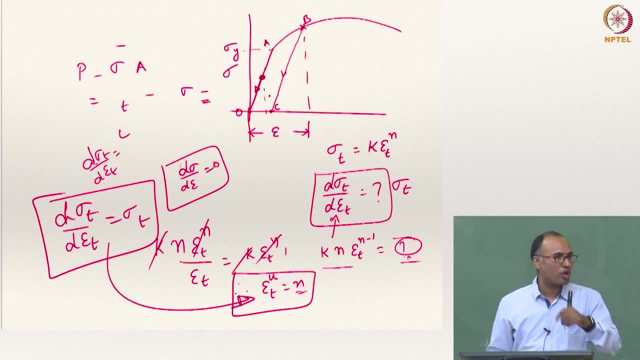 means I have no to zero stress. I could actually go in the opposite direction, but I am not talking about it. zero stress- Then what happens? Because of the fact that I have gone into Plastic regime, I am not able to get to this point where I have actually started, right? 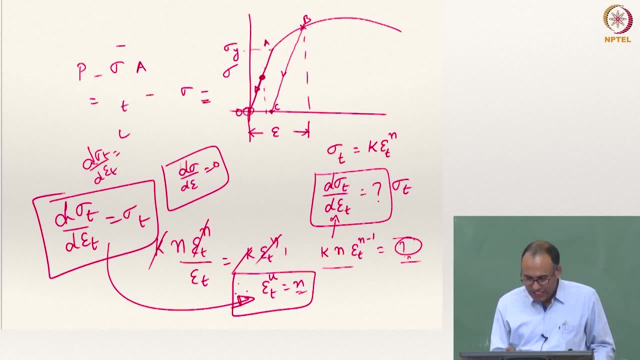 So what happens here? So what is the amount of strain that I have recovered? this is the total strain, but this much strain is recovered right And this much strain is retained. So what should I call this guy? and what should I call this guy? 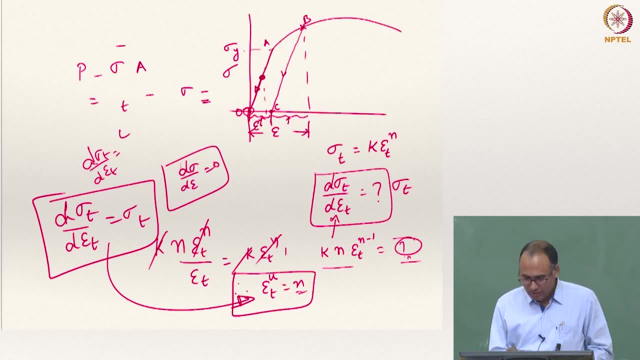 Which one is plastic, first one or second one. So this is your plastic strain. Okay, So this is your plastic strain, this is your elastic strain. So your total strain is given by elastic strain plus plastic strain. is that clear? So now I have unloaded, I had my tea, and then come back. 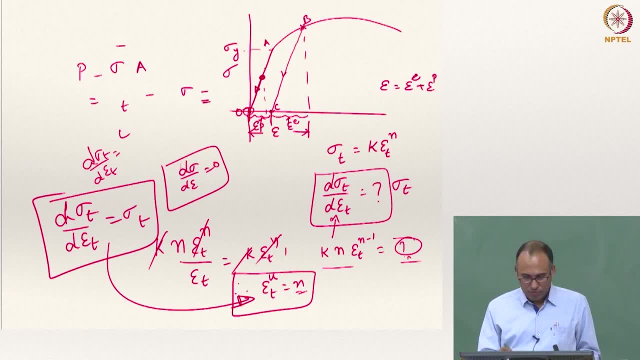 Now, if I start to reload the machine, take the sample which is unloaded up to here Now I am doing the experiment again- how will it start loading now Along the same line? okay, and it will go up to what will be the yield strength of this. 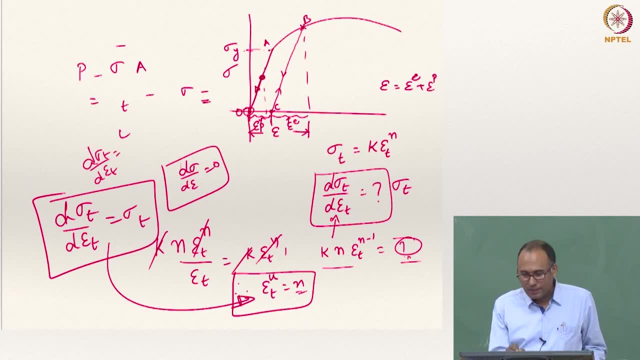 material. Will it be this or that? What happened to the material? You have got the same material right. Did you change the material? It was the same specimen. But now, if you do this experiment, you are observing that. So what is the yield strength of this material? 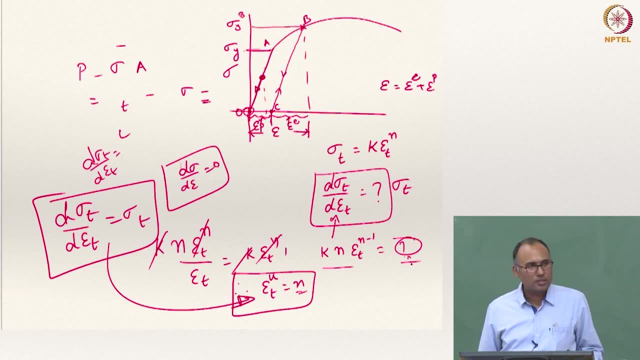 What is the yield strength of this material? The material has a different yield strength. How is this possible? So the most important point to realize is that when we are moving along each and every point on that line, you are actually transforming your material. 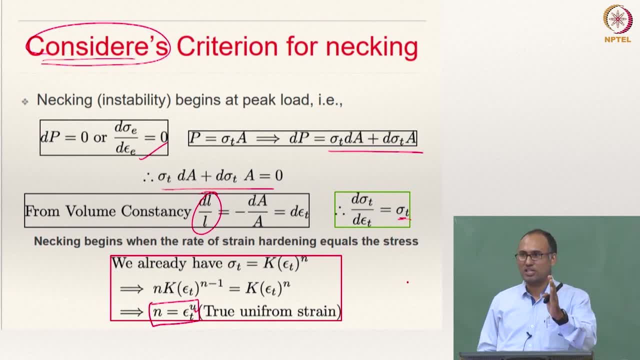 It is not the same material anymore. It may have same elastic modulus, but it definitely does not have same elastic modulus. The yield strength has changed. You have actually changed the material for good by doing plastic deformation. That is why we say: by doing plastic deformation you are hardening the material, right. 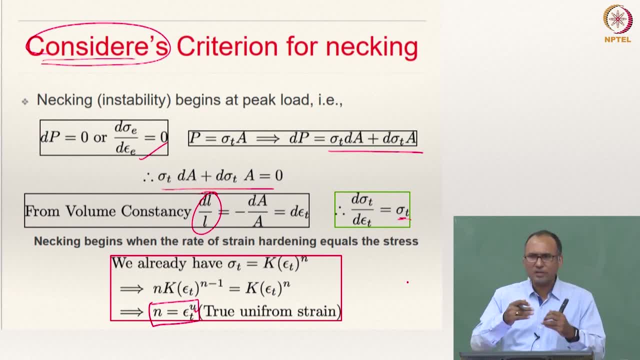 So if you are given a material which is loaded to plastic plastic regime and unloaded, and if you are given that specimen and if you are trying to find out the yield strength of the material, you will find that to be more than what it would have been for a virgin. 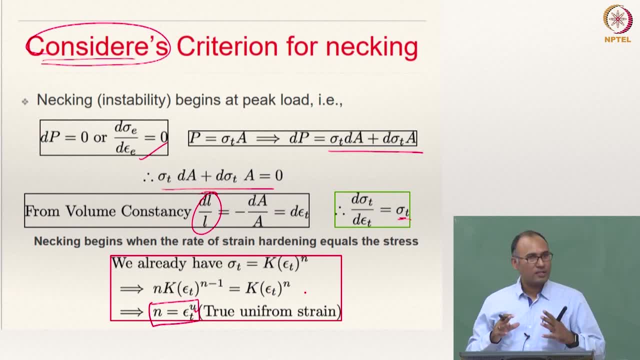 material. So by plastic deformation you are hardening the material Right? So if you take that specimen, is it going to be more brittle compared to the virgin material or not? You will find that it is getting more and more brittle because it is actually going.